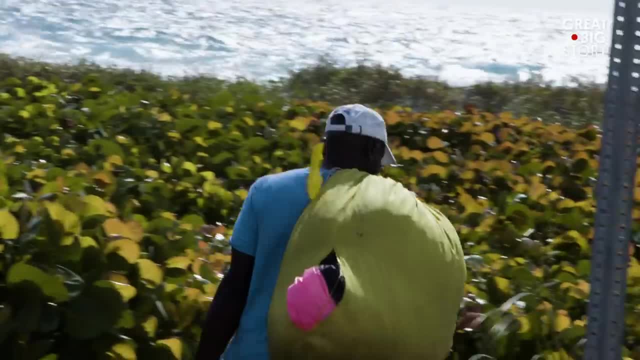 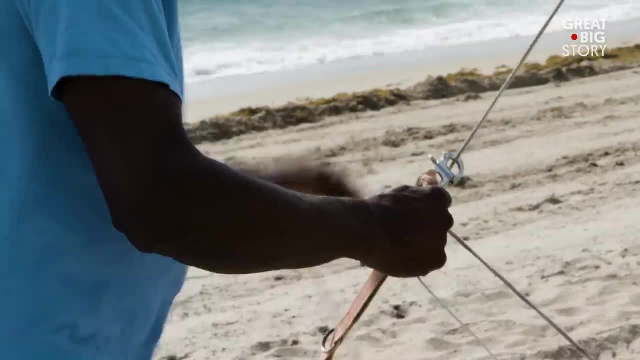 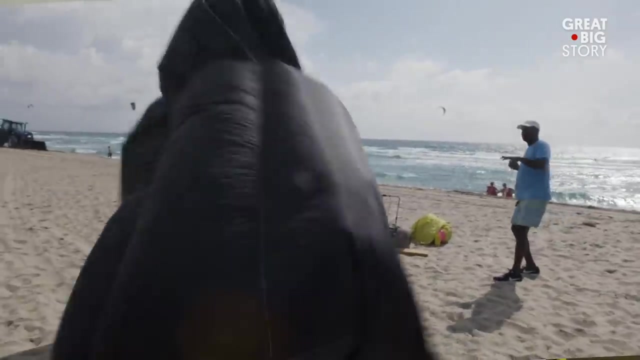 one of the things that I try to take advantage of. Instead of doing it in the classroom at desk, we take them out in the field. The Pythagorean Theorem is a formula used to determine sides of triangles. If you want to use the Pythagorean Theorem on a beach, as we're trying to fly a kite and we let 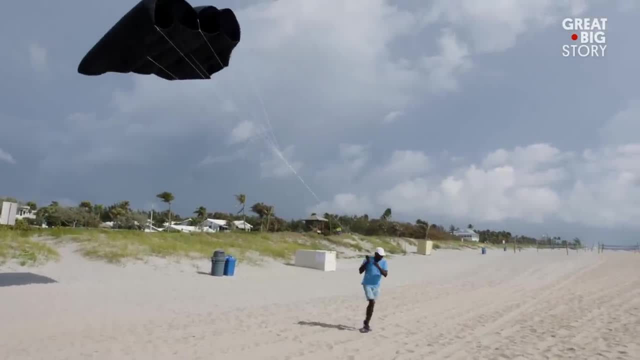 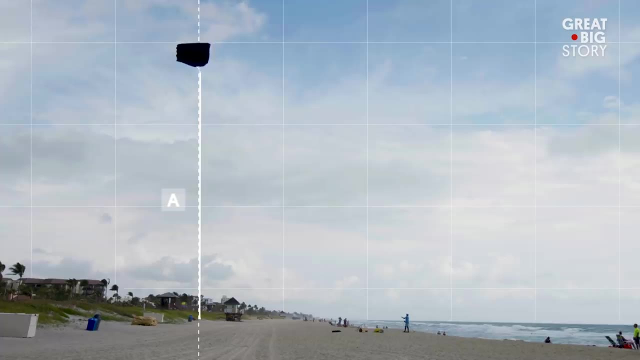 the kite go and it travels up the line better known as the hypotenuse. If we draw a line from the top of the kite down to the bottom, that's side A. If we draw another line from that point back to where we let the kite go, that would be side B. 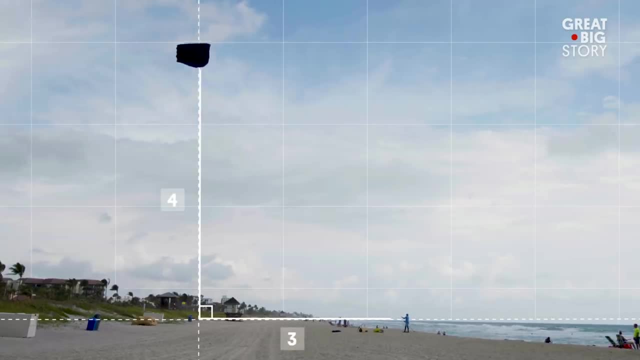 So by plugging those numbers in to the triangle, we have just figured out how long our string is from where we are standing to the top of the kite. Make sure that's a frequent fraction. Common denominators, uncommon denominators, The more. 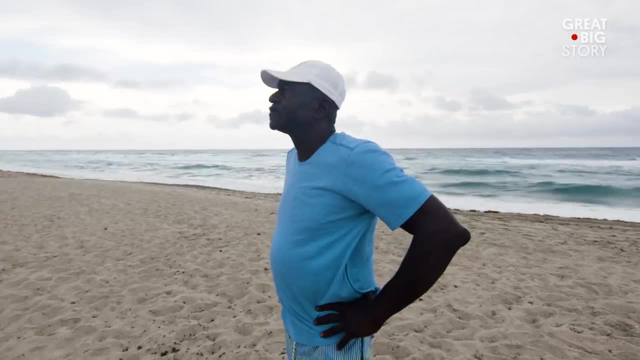 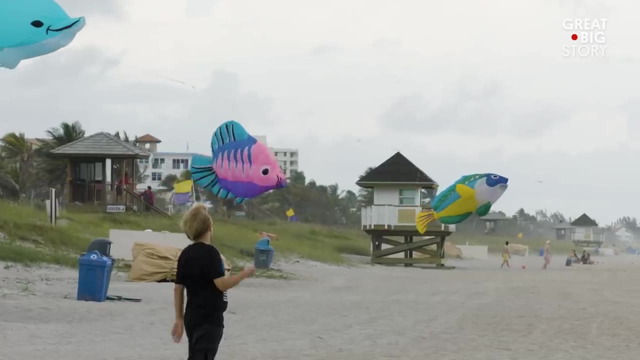 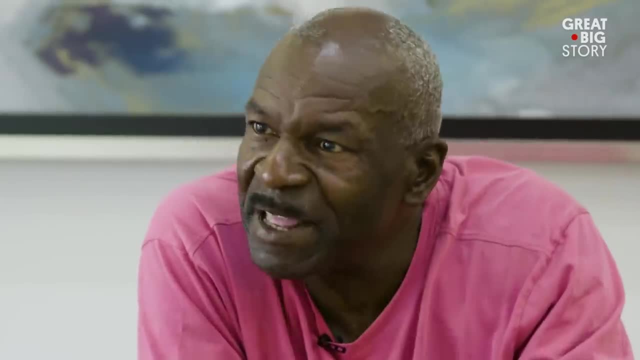 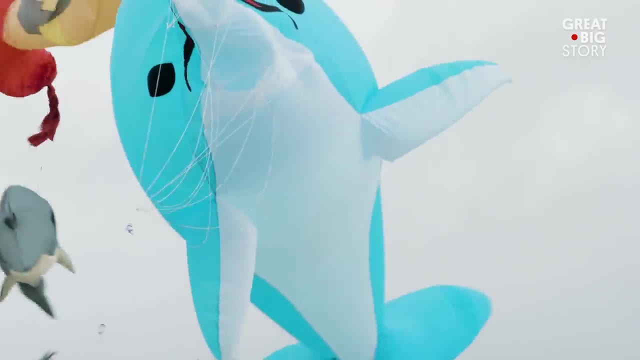 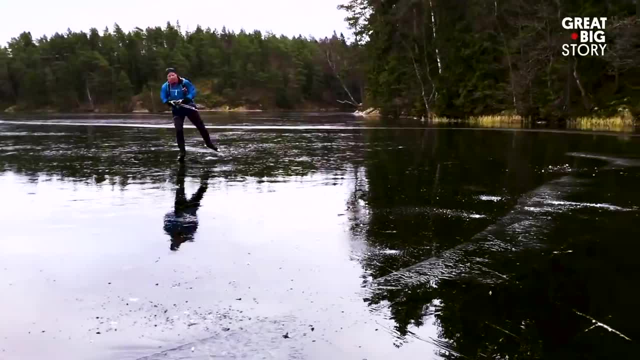 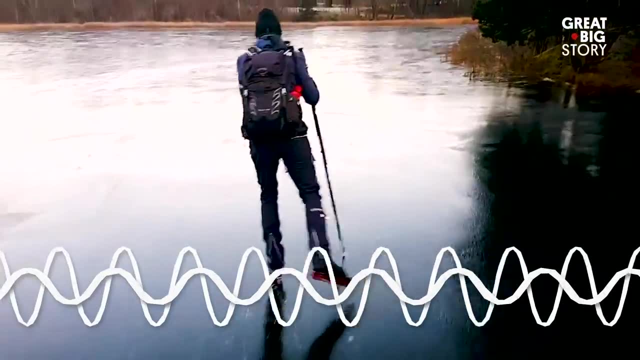 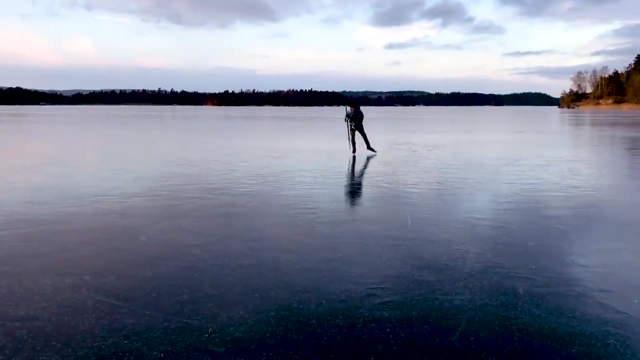 The ice is typically around five centimeters when I skate on it. That sound you hear is actually a combination of two sounds: It's the sounds from cracks striking beneath me and the vibrations within the ice plate itself. It sounds like it's something supersonic. 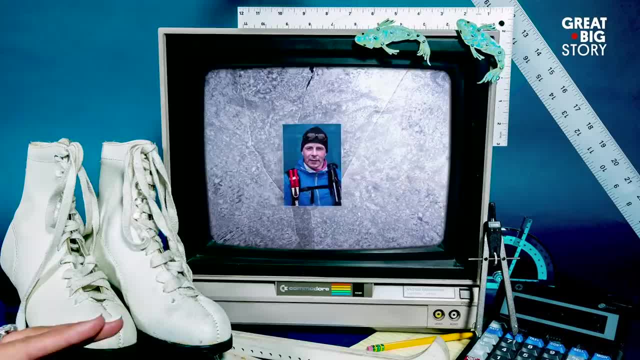 Meet Morten Einer. Hi, I'm Morten Einer. He's a mathematician who enjoys riskier hobbies than most. He's a mathematician who enjoys riskier hobbies than most. He's a mathematician who enjoys riskier hobbies than most. 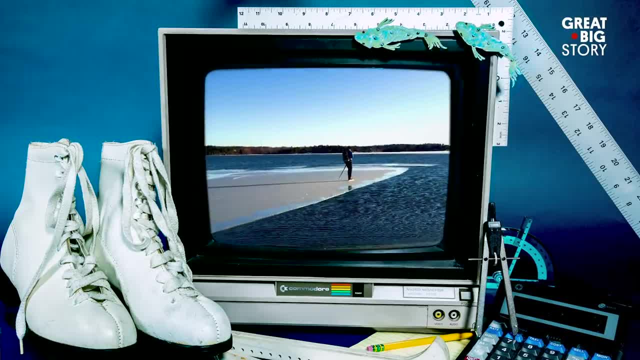 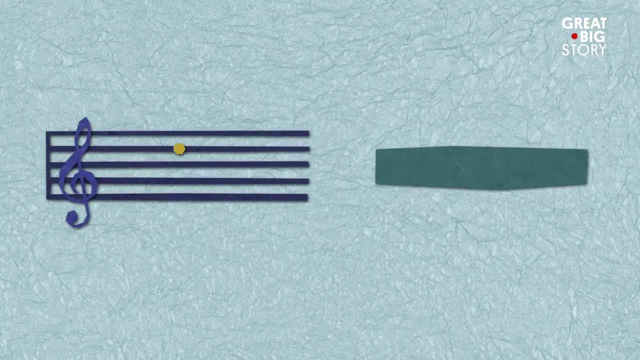 I've been skating on thin ice for 40 years. I've been skating on thin ice for 40 years. When he's skating, though, he's also listening. When thinner the ice, the higher the pitch, Just about when the ice is to break, and that. 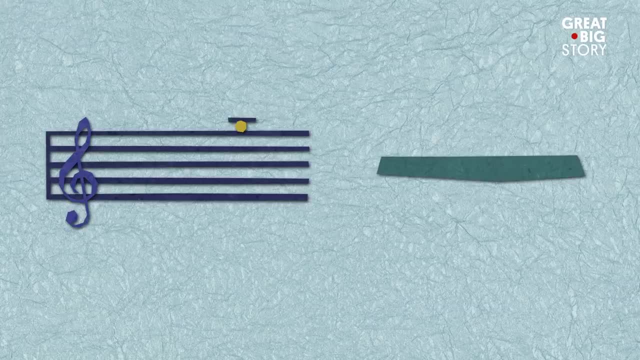 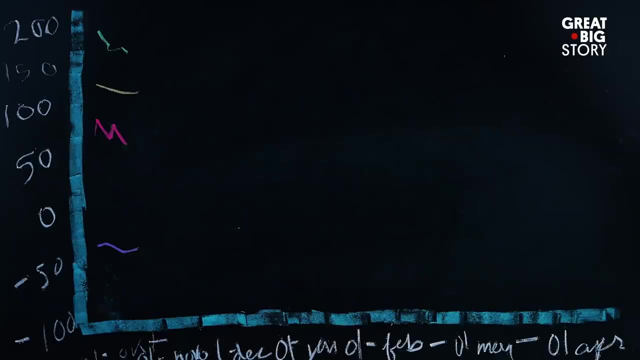 would be about three centimeters. the pitch is at the highest C, the supposedly highest note of the soprano. C Morten relies on his knowledge as a mathematician to calculate the thickness of the ice, its flexibility. to calculate the thickness of the ice, its flexibility and its temperature. 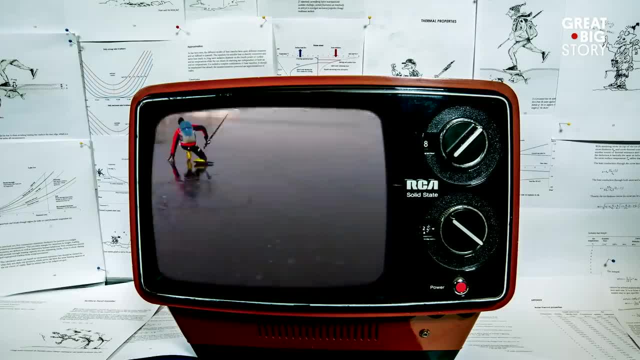 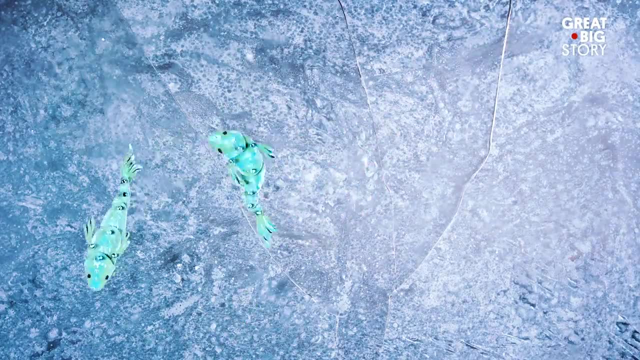 Skate. people tend to freak out when they see us skating on thin ice, but I couldn't be more calm because I know what I'm doing. Sometimes the ice is perfectly clear and I can see fish below even a beaver, and also freed divers swimming under the ice. 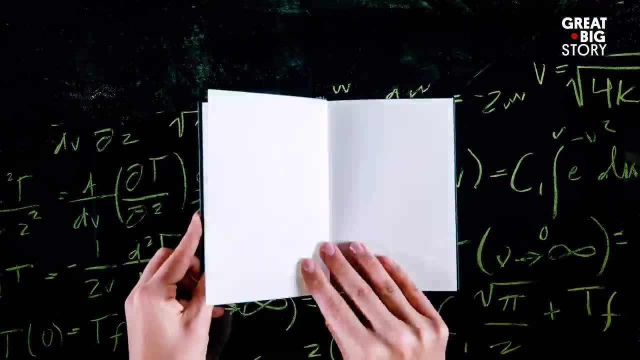 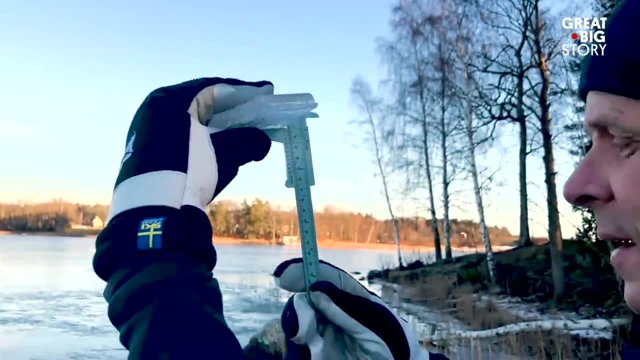 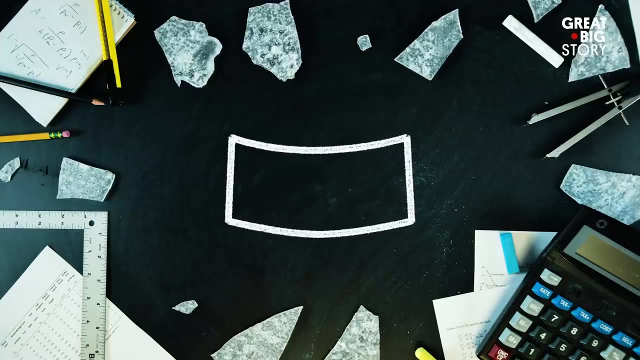 When Morten first started, there wasn't any physics or scientific information to explain how thin ice skating is possible. He studied the ice for 10 years every winter to explain the phenomenon. I observed three things with a thin ice. One is that the ice bends, and the thinner it is, the more it bends. 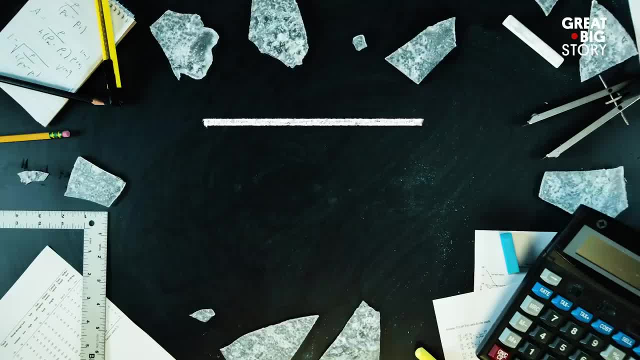 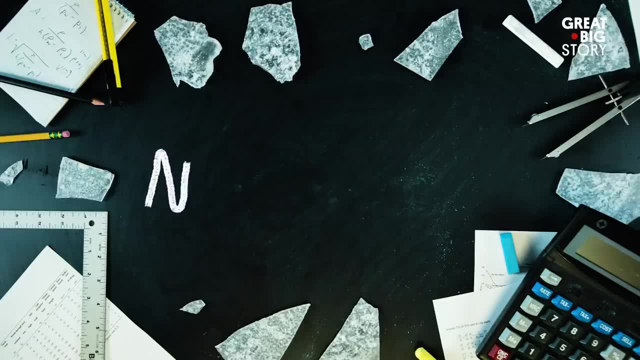 The ice needs to be flexible to support you. Second, the first crack is a true warning signal. then I know the ice is thin And when it gets even thinner, more cracks evolve. And finally the ice gives sonorous tone, beautiful eerie tone, which immediately tells: 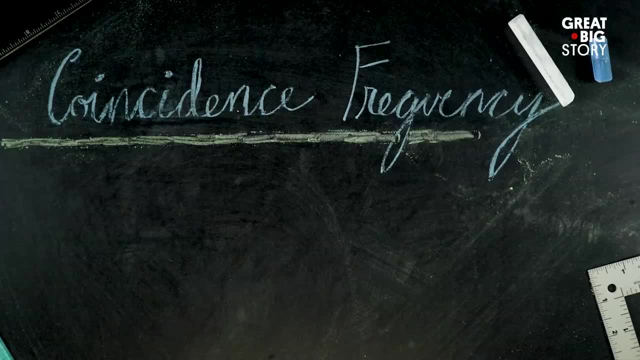 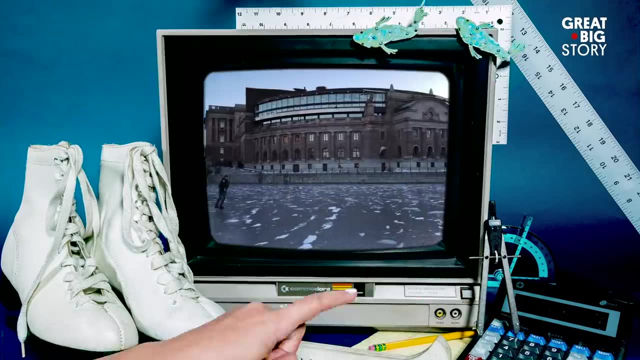 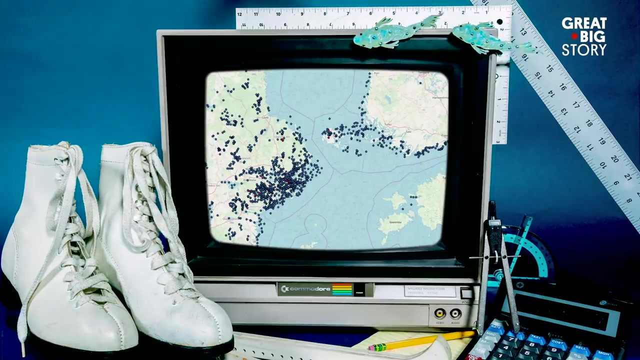 me how thick the ice is. It's called the coincidence frequency And it can be calculated mathematically. Morten has skated on over 1,800 bodies of water in North America, Norway and Central and Eastern Europe. I love skating for the excitement and challenges it brings. 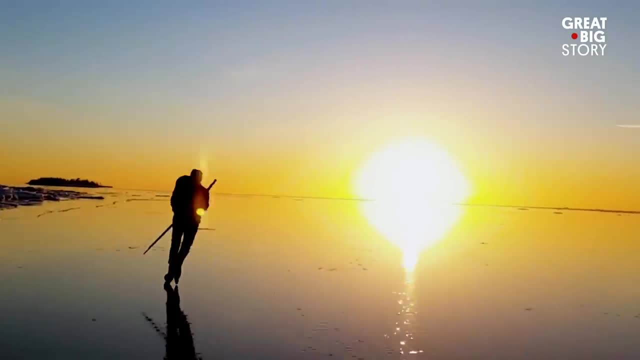 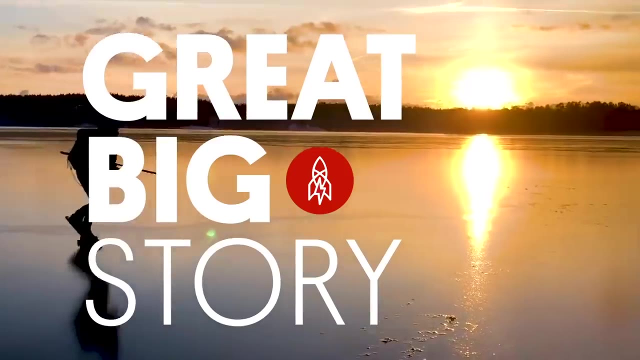 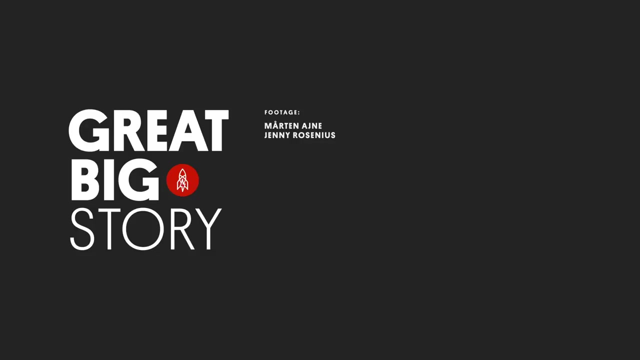 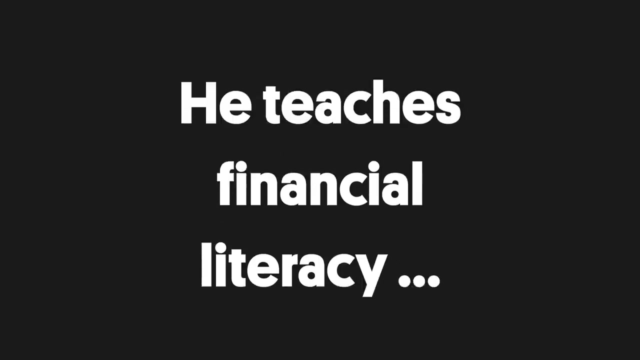 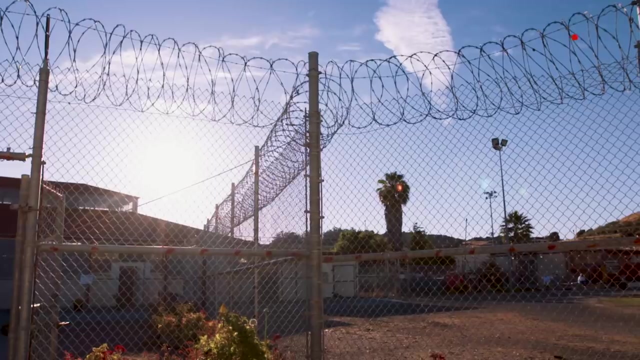 It's an opportunity for math and nature to come together and make it understandable for me. I've been skating most of my life and I always look forward to next winter. We're going to go ahead and get situated. This is the finance program and we always like to see new faces. 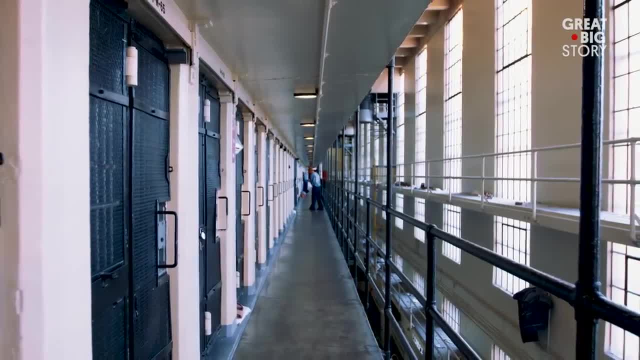 When you come to Wall Street's financial literacy program, you're going to see a lot of people. You're going to see a lot of people. You're going to see a lot of people. You're going to see people in the financial literacy class. 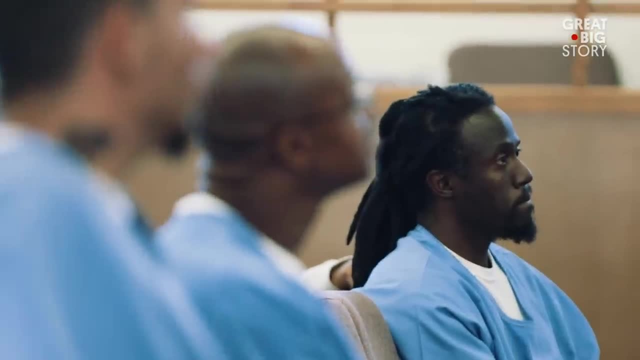 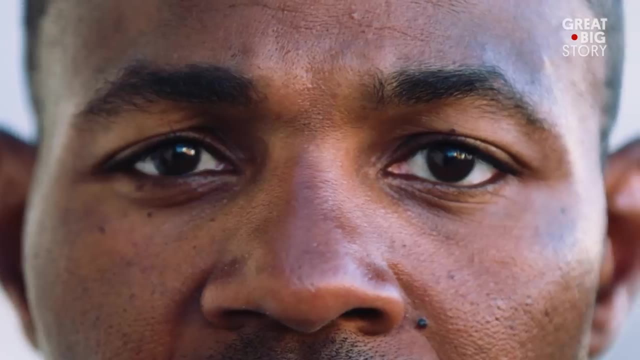 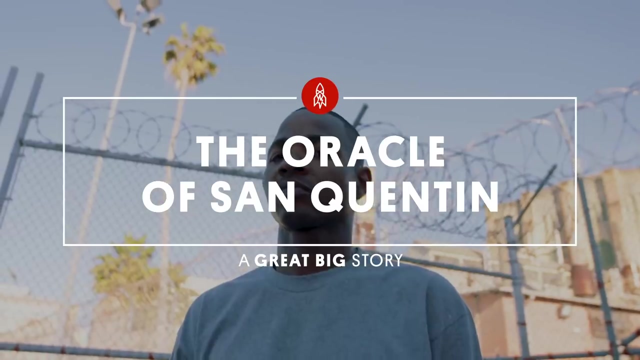 You're going to see people with tattoos and dreads and just people you normally wouldn't expect to see. learning finance. You're going to see people of all different backgrounds looking for hope. He makes it universal. If I tell you, I'll give you the 50 bucks, but I want you to pay me back $50 in interest. 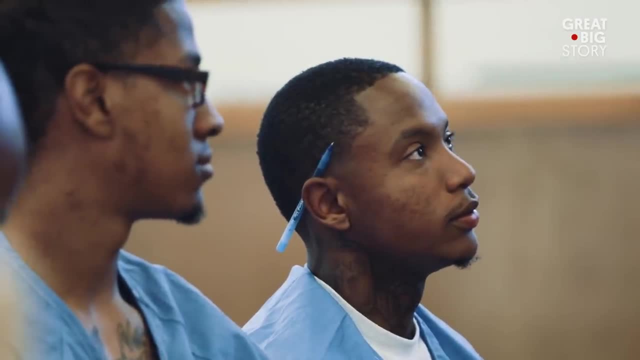 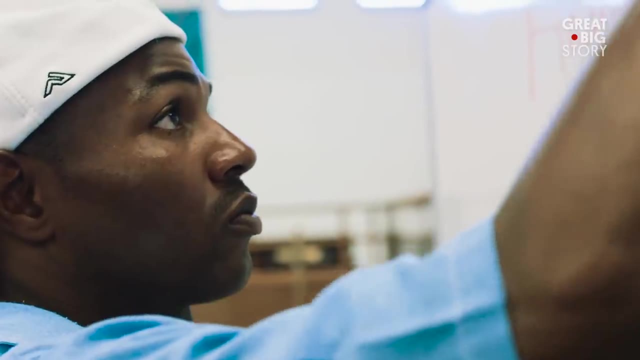 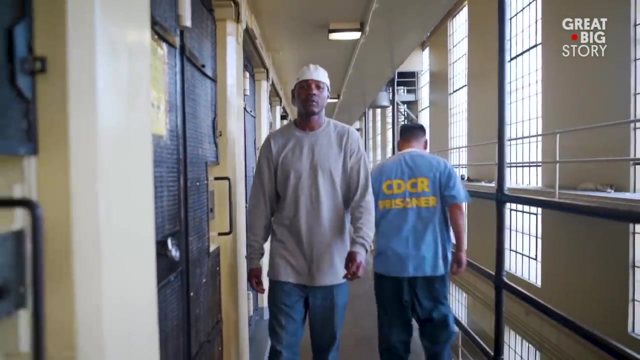 what you going to say. Say no. You going to say what No? And why you going to say no? Why You, looking at me, absorb that one Rights. That's what I asked you to say. No, That's what I wanted to say. 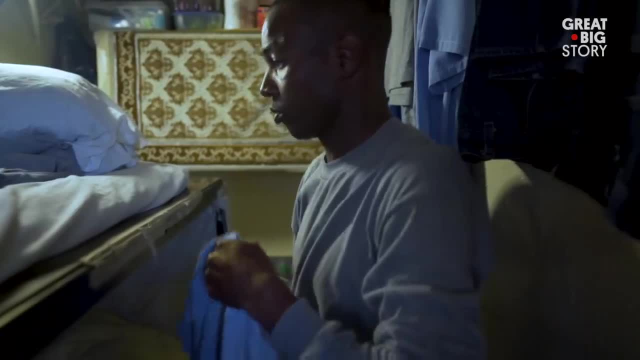 No, That's what I zwe: Full extent. No, No, No. That's not an investment for a huge market provider, That's for, like, a number of styles, like how I live my life. It's not the sale. 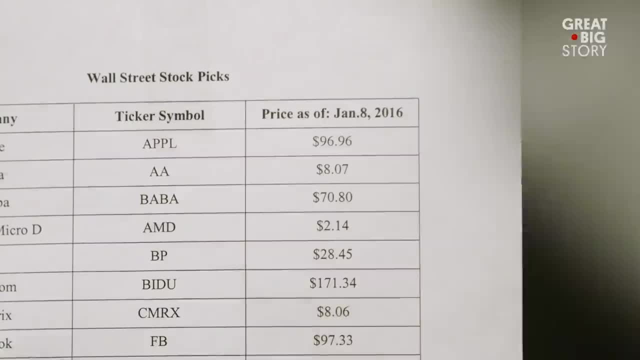 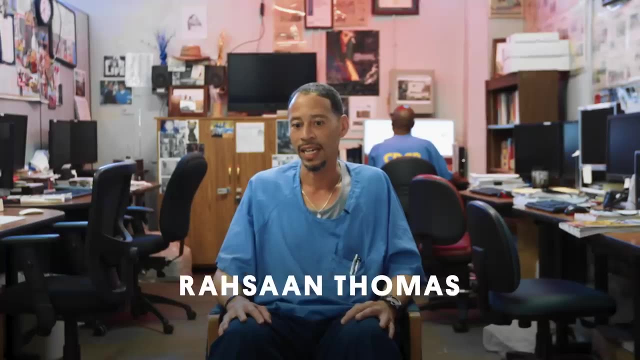 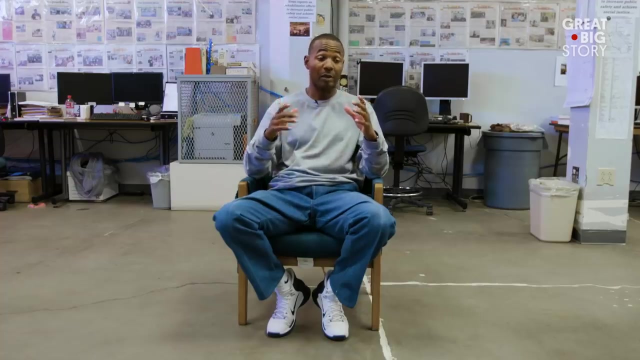 It's like a high school transfer in them, Right, Right, Wow illiterate. He doesn't have a college education to this day, He only has a GED. and yet this guy is successfully trading from prison My cellie who had come from juvenile hall with me. he would read the sports page to me. 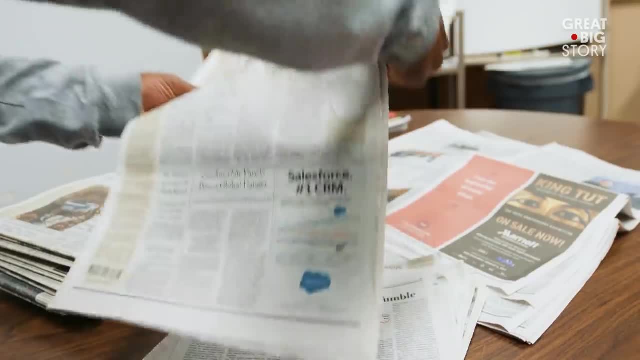 He'd be like: man, go get it and I'd read it. I grabbed the paper and I was like I got it And when I turned around, an older guy said: hey man, you play the stock market. 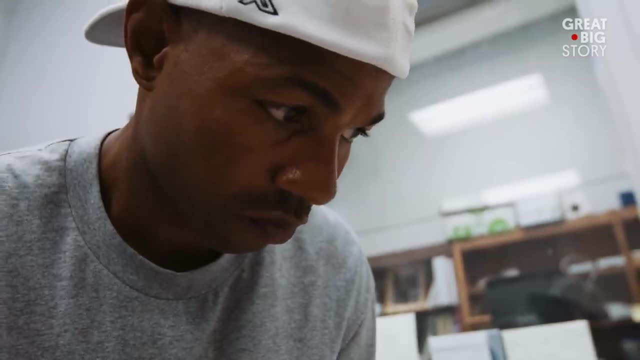 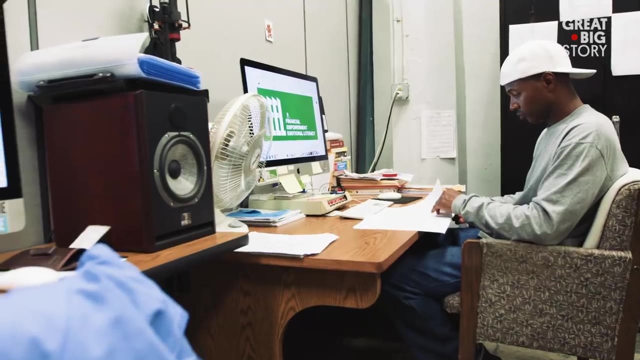 And I realized that I picked up the business section instead of the sports page. I was like ah man. And I asked him what the stock market was and he told me he said that's the place where white folks keep all their money. And that's when I really first discovered the stock market. 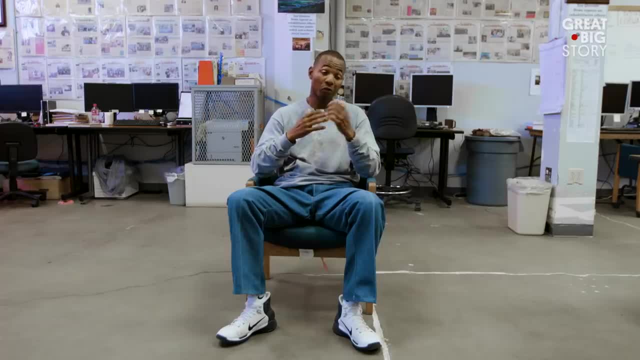 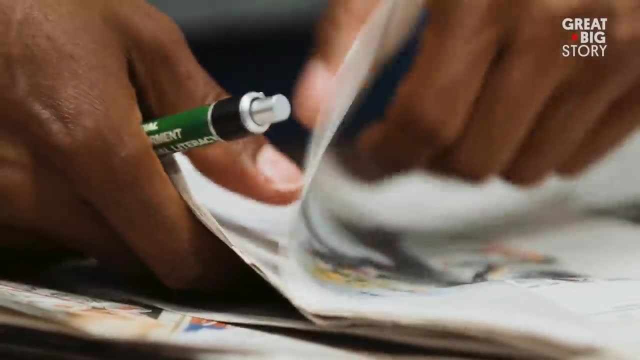 So I started teaching myself how to read. Family and friends on the outside opened up online brokerage accounts and I basically told them what to buy and when to buy and when to sell. And I mean that was just simply because it was really just that easy. 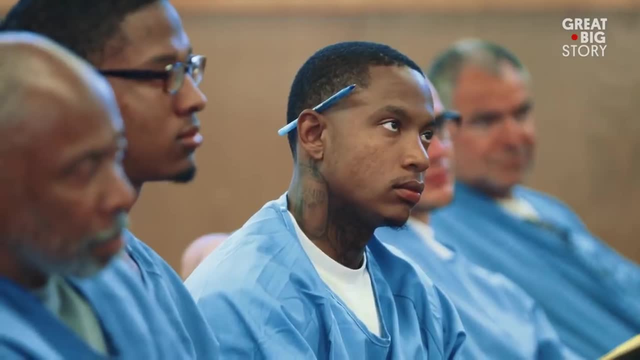 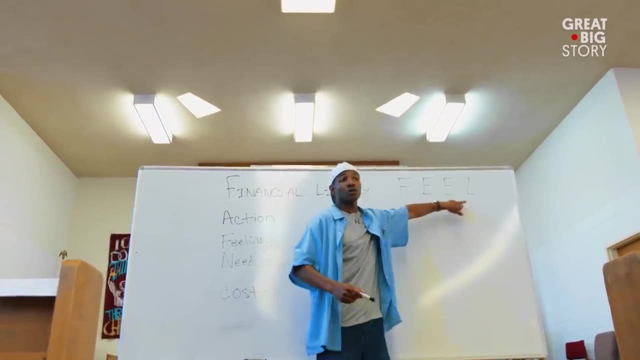 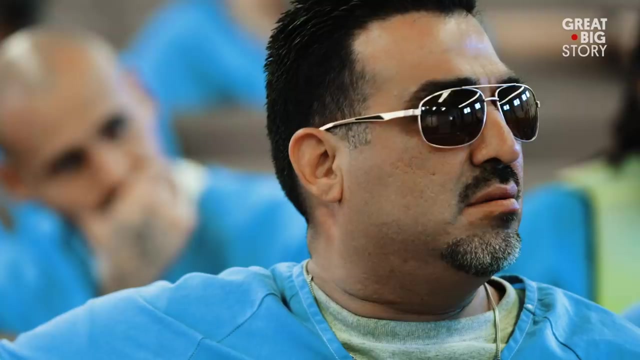 This is a finance program, but I don't teach about finance. I teach financial empowerment, emotional literacy. That's what I teach. So I think financial education is important for incarcerated people, given that the crimes that are committed are financially motivated and driven. 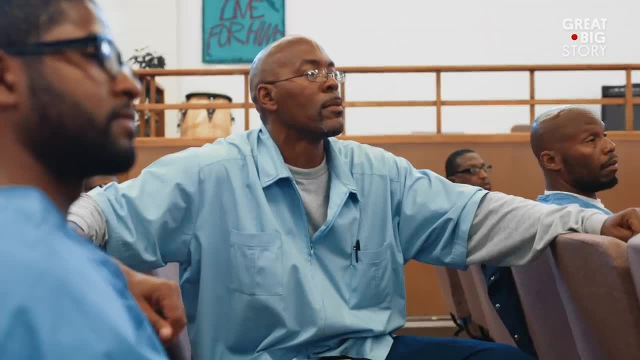 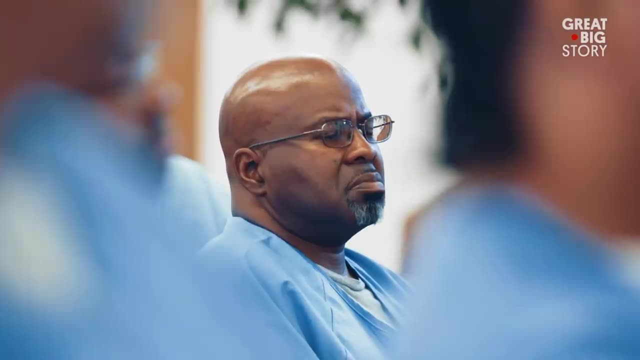 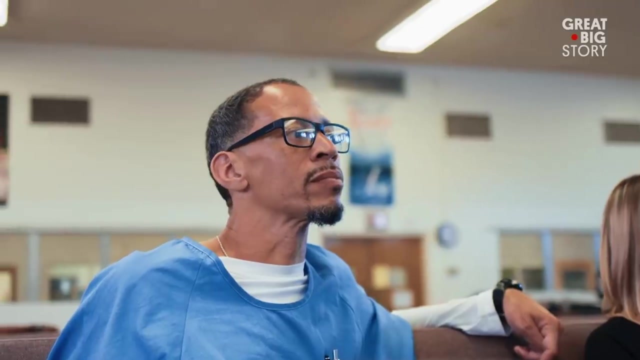 When I learned about financial education myself, I thought that would be something that other men in my same situation could benefit from, And so now the program teaches incarcerated men how to better manage their emotions in relation to their financial standing. So you got to weigh your strategies. 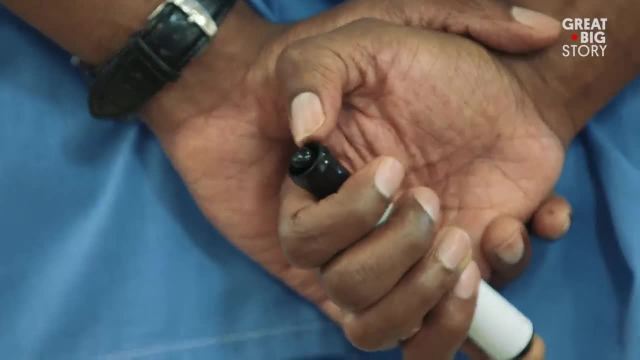 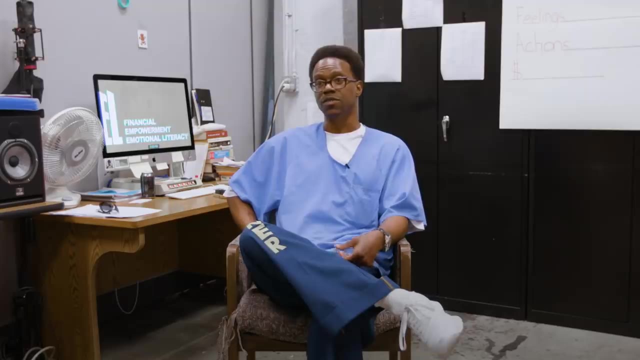 when you're talking about giving yourself room to start saving money. When you're traumatized, you do a lot of things. you don't know why you're doing them, And that happens with finance too. I suffered a lot of trauma in my life, and my trauma like culminated in me murdering a man. 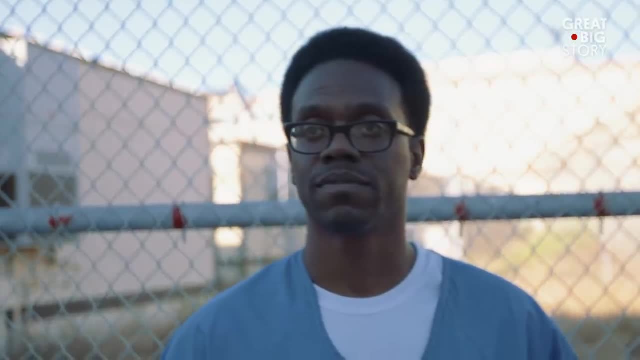 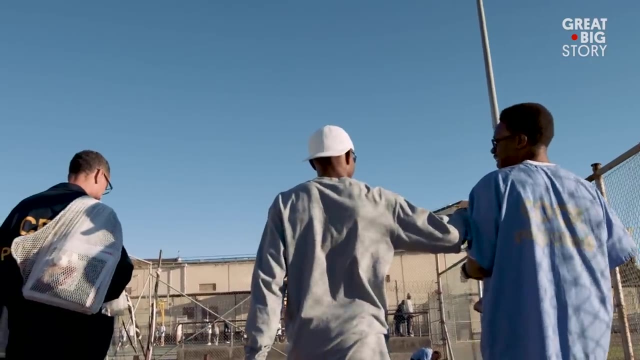 So, while this is very important to me, because I do need to manage my money and manage my life, What's most important is that I'm managing my emotional responsibilities, because the last time I didn't do that, a man lost his life. I don't think you can have full rehabilitation. 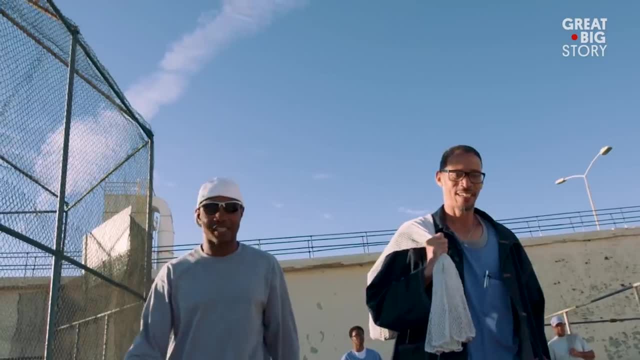 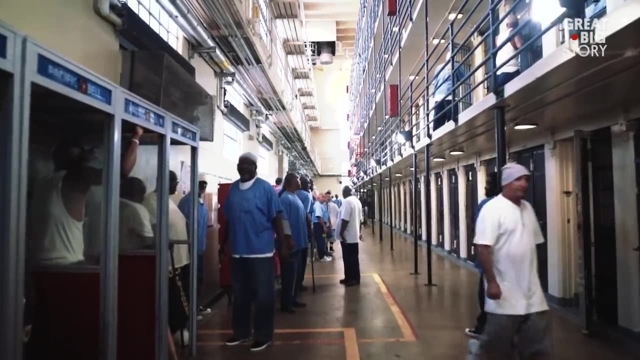 without financial education. I can make amends for the crimes that I've done. I can even stop doing the things that I've done, But I think for people who were criminals, when you empower those people and they know that they don't have to commit crime, 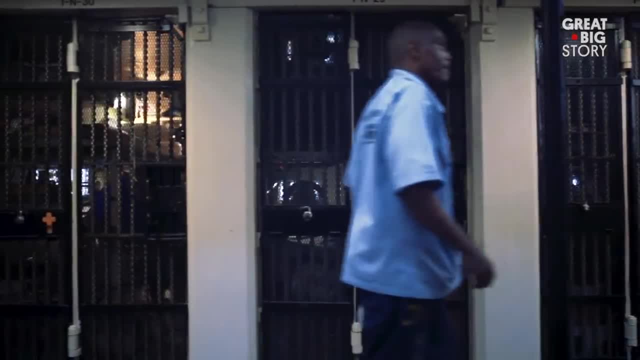 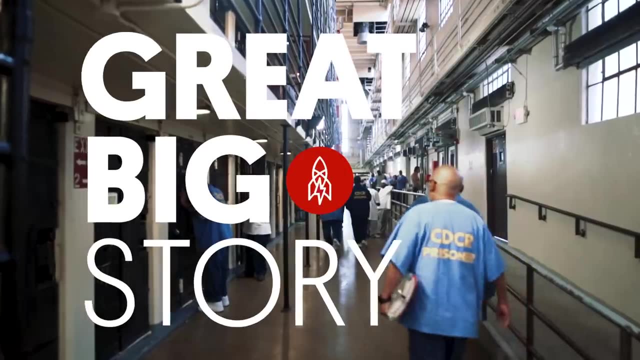 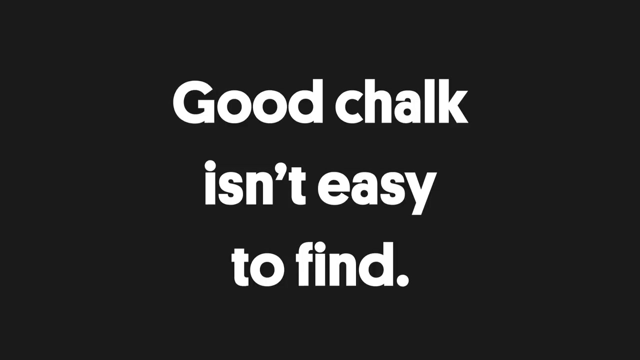 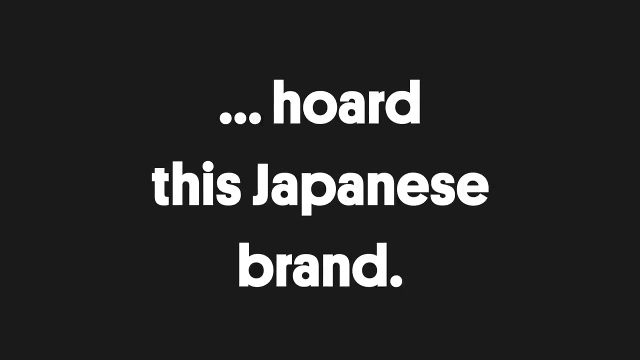 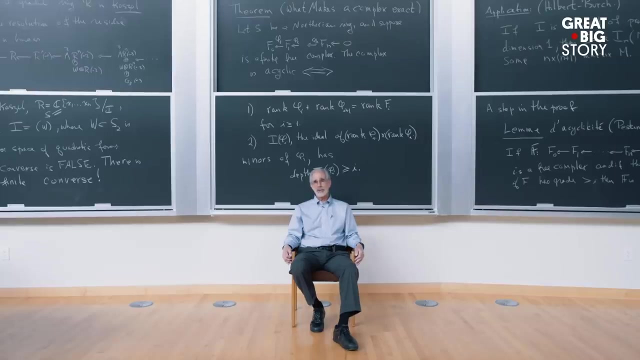 like I did when I learned that I didn't have to commit crime. it was like wow, like I can really make something in my life and now I don't have to be a criminal. The legend around this chalk is that it's impossible to write a false theorem. 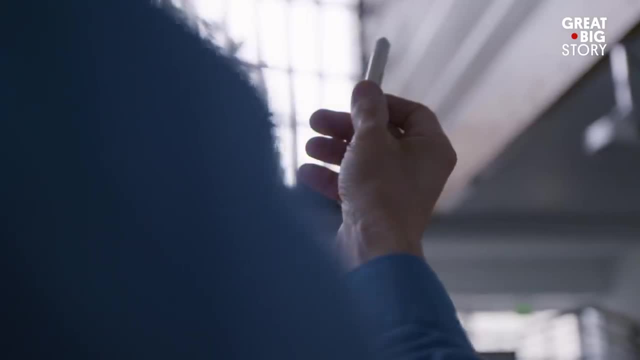 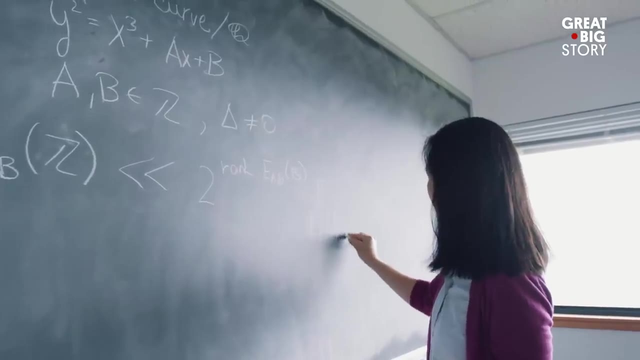 I assume the special ingredient was angel tears. Mathematicians from all the top schools very frequently use it. It's a cult favorite. As soon as I used it, I was a convert. The chalk is one of the best kept secrets in the math world. 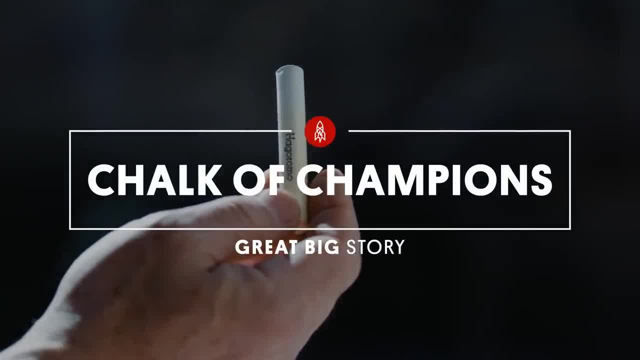 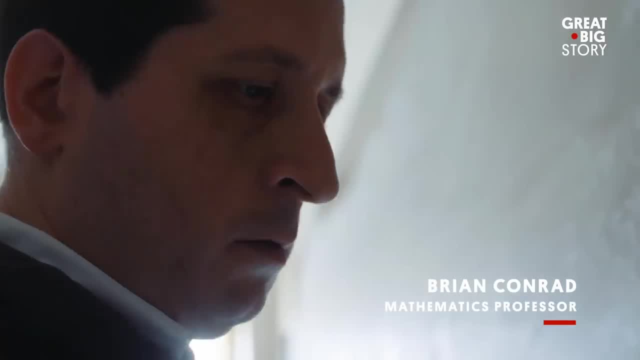 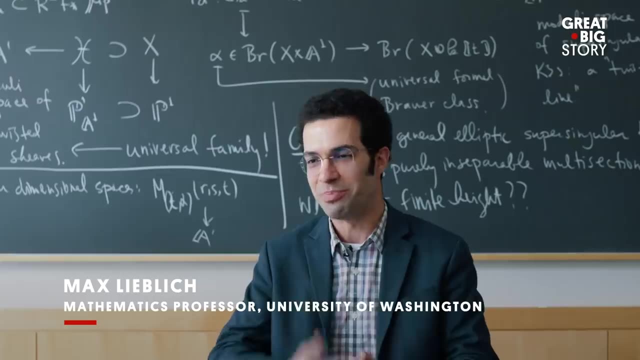 It's the Rolls Royce of chalk. Hagoromo is a brand of Japanese chalk. The way it flows on a board is a bit hard to describe in words. It's really hard to get. You can only get it from Japan. You need a Japanese person to bring it back for you. 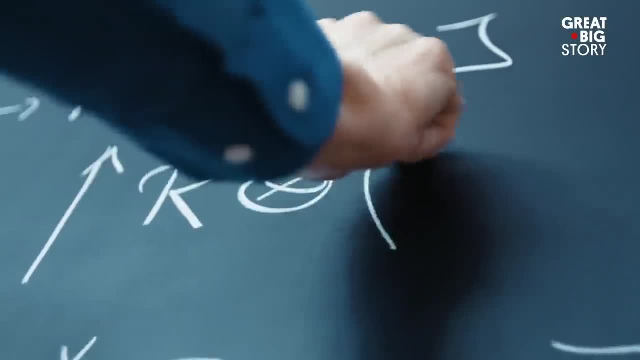 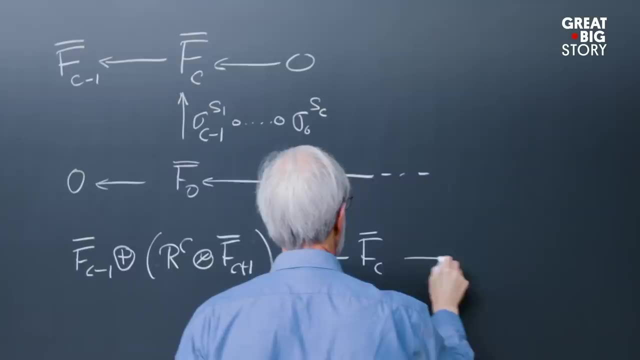 I discovered it when I went to visit the University of Tokyo and one of the professors there said to me: you know, we have better chalk than you do in the States. And I said, oh, go on, chalk is chalk, And so I tried it out. 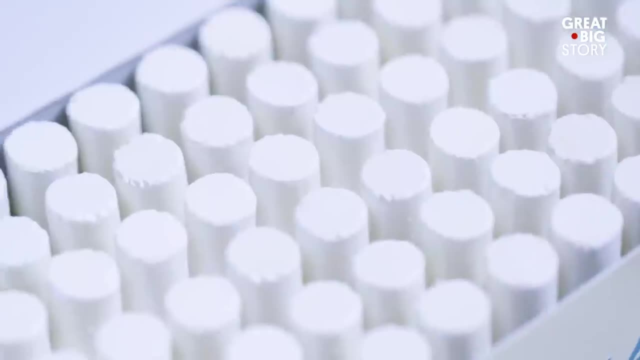 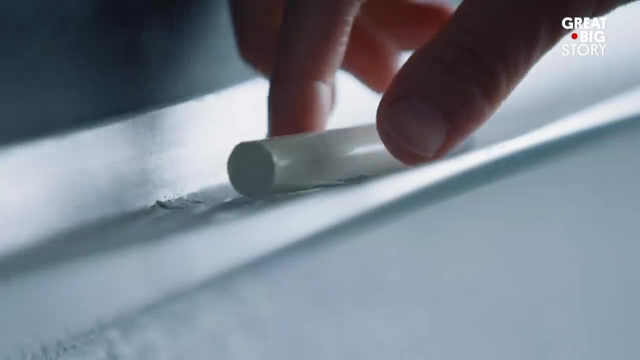 and I was surprised to find that he was right. I tried it and I thought it was phenomenal. It's the densest, it erases the cleanest, it leaves the nicest line. If you use bad chalk often you have to press really hard. 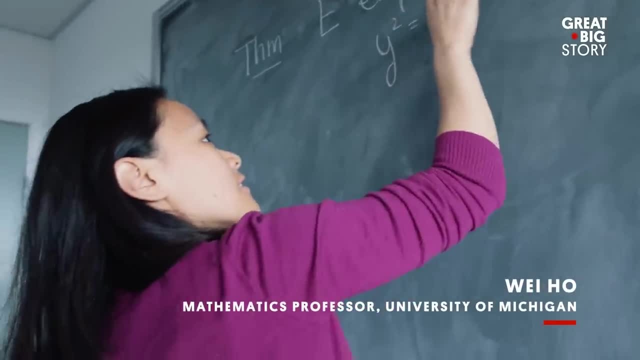 and you have to press really hard and you have to press really hard for anyone to see what you're writing. So, using Hagoromo on a good board, it doesn't really feel like you're working hard to write. When I'm teaching, I get a feeling of energy. 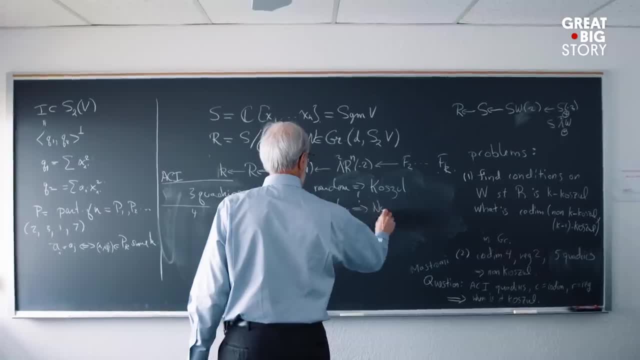 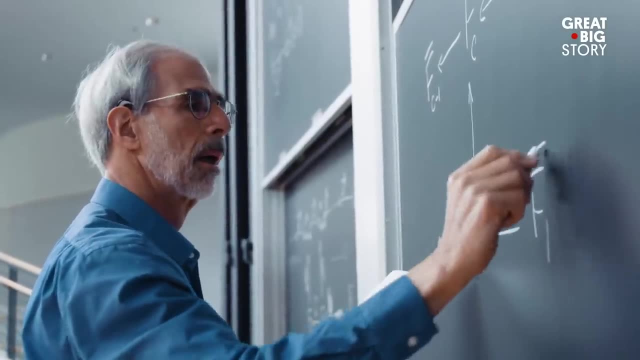 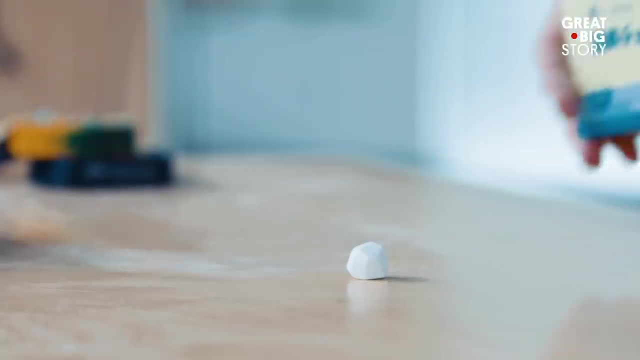 confidence, and the chalk absolutely helps. Slowly the math world has become aware of this and it became a bit of a fad in some circles. It was like maybe four years ago the word came out that the company was going out of business. 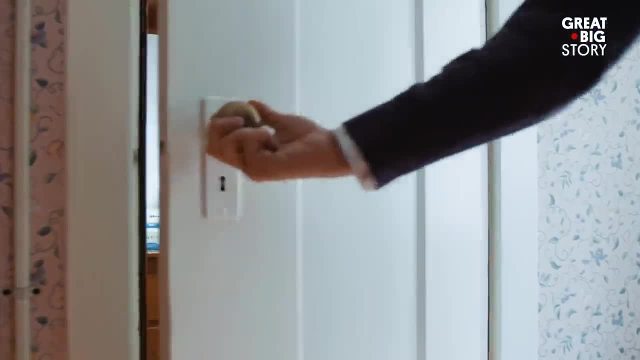 It was like maybe four years ago, the word came out that the company was going out of business. I sort of jokingly referred to it as a chalk apocalypse, so I immediately started hoarding up as much as I could. I ordered three boxes of Hagoromo. 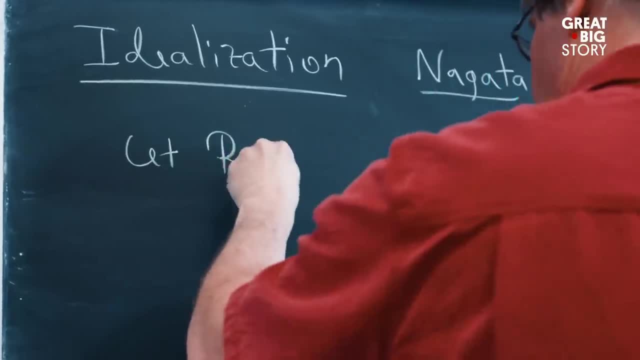 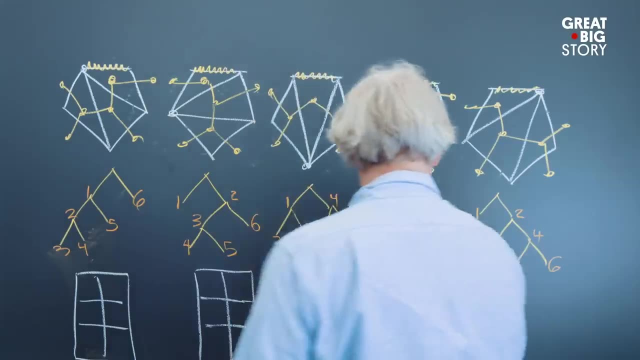 and kept it in my office and used it very sparingly. I should have bought more, but I have friends that bought boxes and boxes and boxes of the stuff. They might very well be set for the rest of their career. We got like 1,500 sticks. 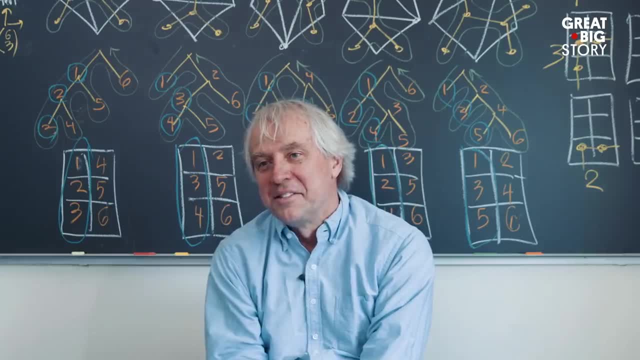 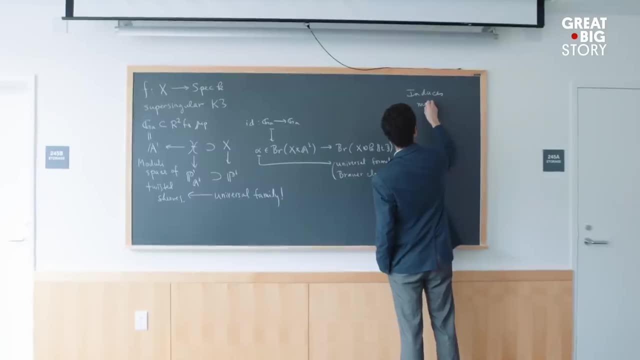 That's a lot of days. four sticks a day. I think I'm gonna make it. I have probably a 10-year supply still at home. I calculated how many boxes would I need to last for 10 years- 10 or 15 years? 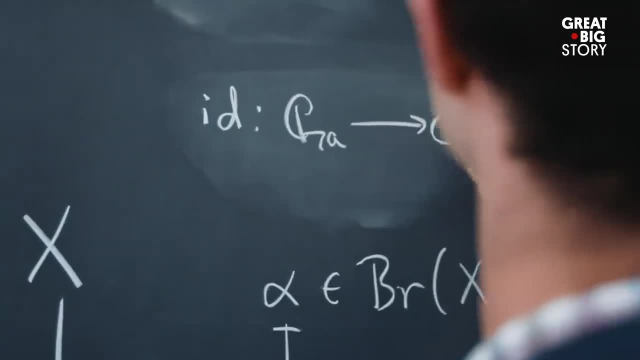 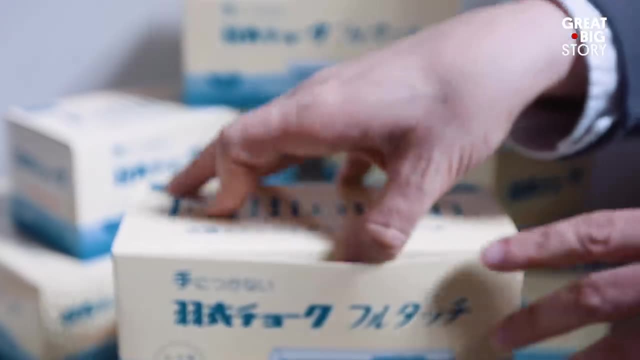 I didn't want to become a chalk dealer, but I did like the idea that I could be the first stick-is-free chalk dealer on the block in my department. I was probably selling it regularly to maybe eight to 10 colleagues. I would reach into my cupboard in my office. 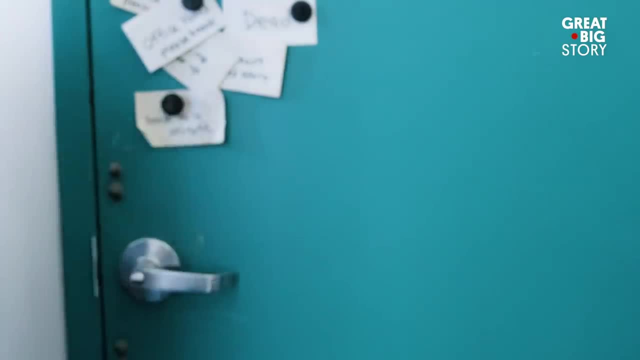 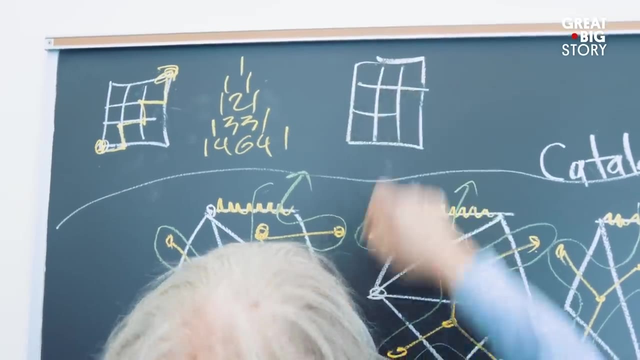 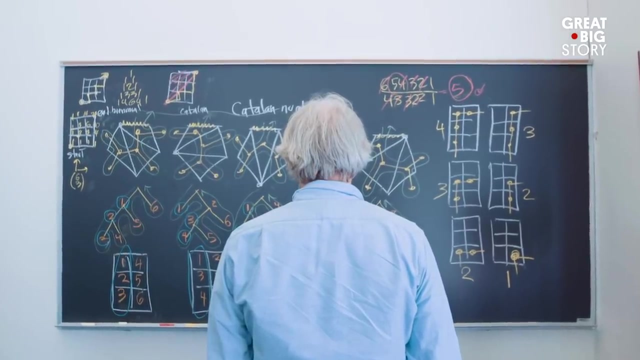 and pull out another box and we'd do the deal. in my office We all had a chalk fix and we still do. The original Hagoromo chalk is slowly disappearing. A few years ago a Korean company bought their formulas and did the best job of faithfully reproducing it in Korea.